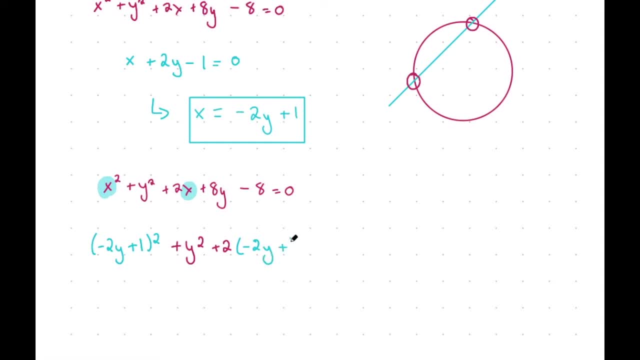 2, and I'm going to replace that with x, and then I'm going to put in a point of intersection: by minus 2y plus 1 plus 8y minus 8 is equal to 0. so then I'm going to square that out and I'm going 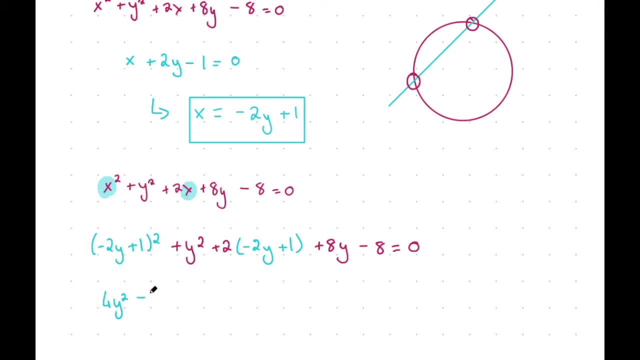 to get 4y squared, minus 4y plus 1, then I'm going to have the plus y squared next, so plus y squared, and then I'm going to multiply this out, which is going to give me minus 4y, and then I'm going to 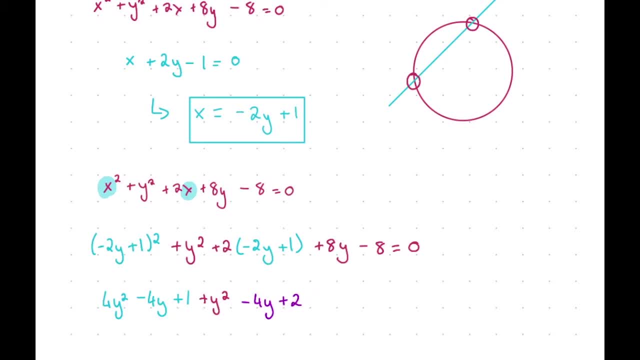 have plus 2 and then my plus 8y and minus 8. so plus 8y, minus 8, and all of that's equal to 0. so now what I'm going to do is tidy it up where possible. so I'm going to have 4y squared plus y. 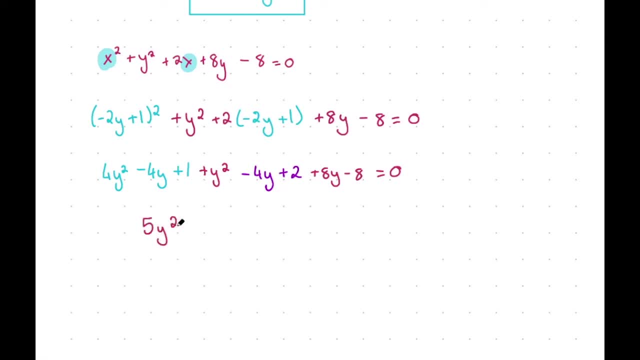 squared. well, that tidies up to give me 5y squared. then I'm going to have 4y squared plus y squared, minus 4y. minus 4y is minus 8y, plus another 8y then is going to give me 0. so all of those. 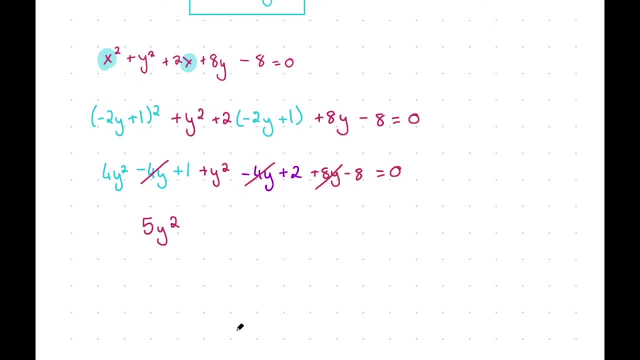 actually add up to give me 0, and then what I'm left with is plus 1, plus 2, which is 3, and then minus 8. so that's going to give me minus 5 is equal to 0. so what I do then is I go through. 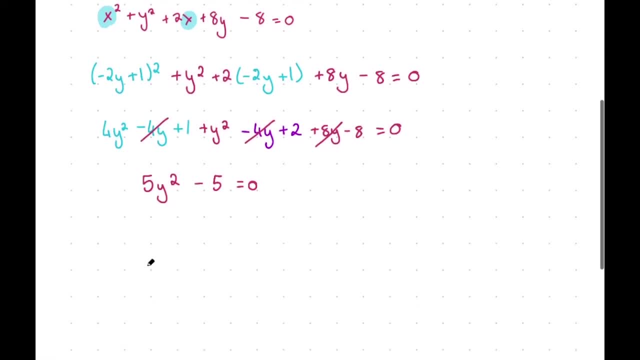 my list of questions when I'm trying to solve anything in algebra and the list of questions is first and second and then I'm going to add up to 0, and then I'm going to add up to 1, and then I'll tell you what I know first. does it have any factor in common and we can see here that? 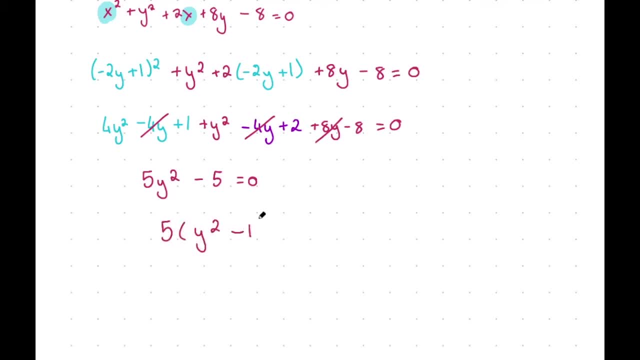 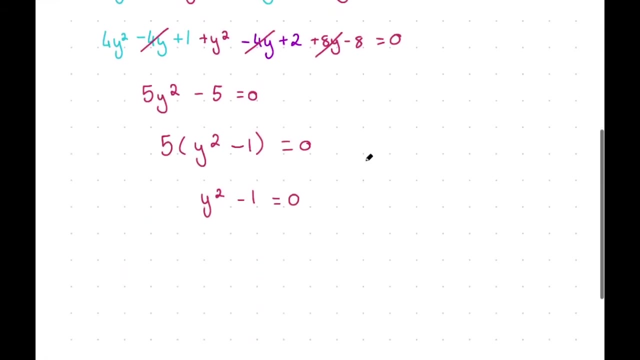 five is actually a common factor, so I can factorize out five here, and then I can say: divide both sides by five and I've got y squared minus 1 is equal to 0. now, remember, we're looking for two points of intersection here. so what I have to do here is use actually the difference. 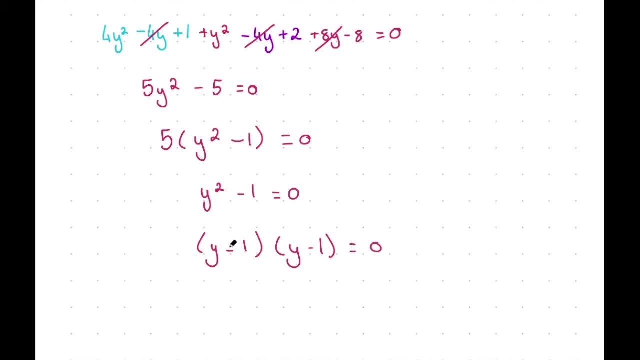 so I'm going to have y plus 1, y minus 1, to give me y squared minus 1, and in that scenario then I get: y is equal to minus 1 and y is equal to plus 1, so I get two values for y. now what I need.